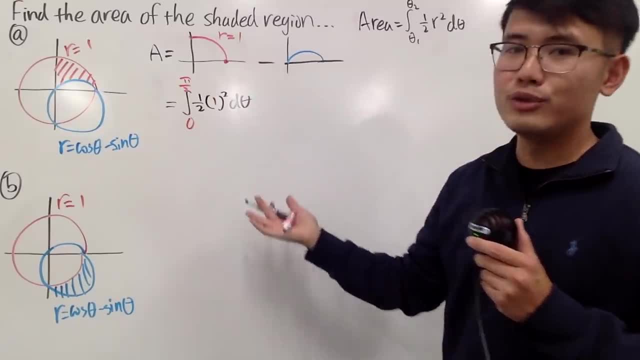 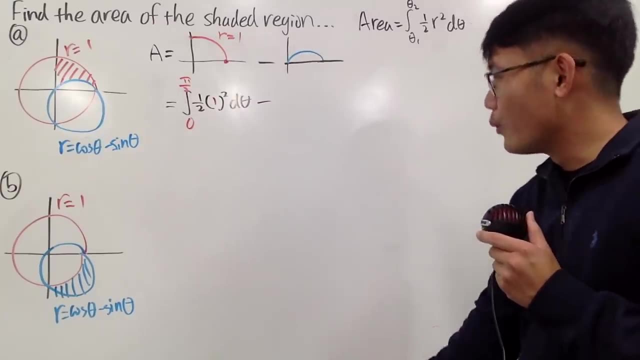 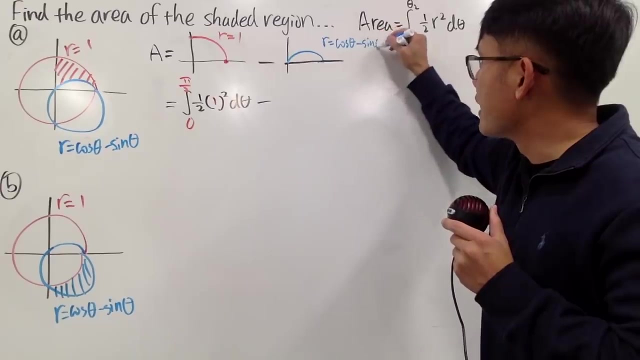 And you square that, and then you have the d theta. Congratulations, we are done- Minus the other part. This part is a tricky part, so pay close attention to this, Well. well, This right here, the function is r being cosine theta minus sine theta. 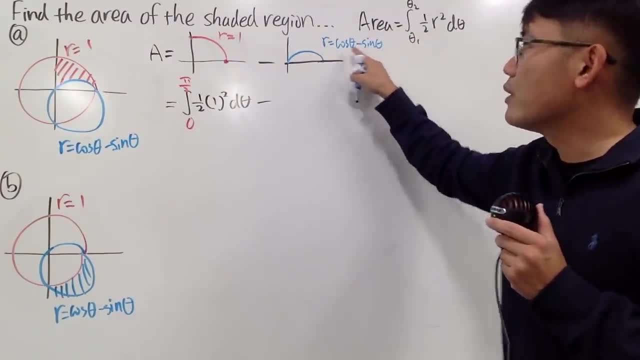 Let me tell you: if theta is equal to zero cosine, theta is equal to zero. Let me tell you: if theta is equal to zero cosine, theta is equal to zero. Cosine zero is one Sine zero is zero. So this point right here is theta one being zero. 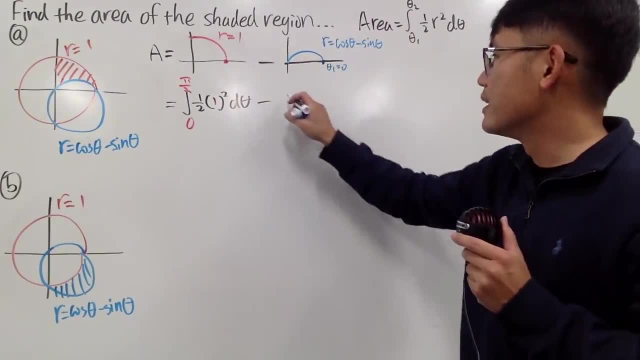 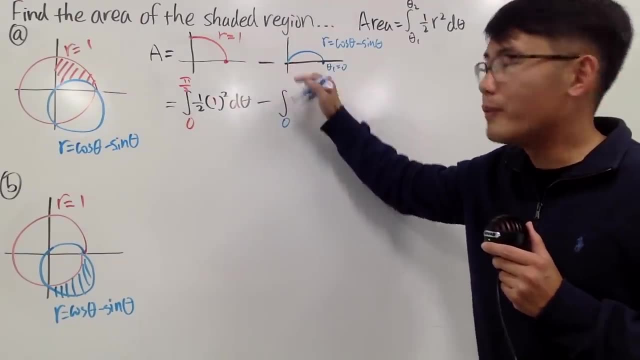 So this point right here is theta one being zero. That's great. So we still have the integral going from zero. That's great. However, we have to find out for what angle will the curve hit the origin. However, we have to find out for what angle will the curve hit the origin. 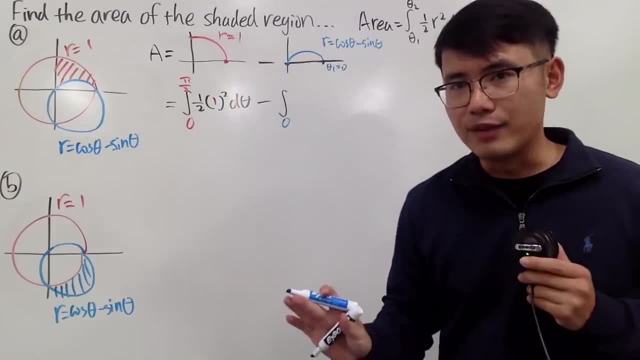 However, we have to find out for what angle will the curve hit the origin? This right here, is not pi over 2, right. Pay close attention to this. This, right here, is not pi over 2 for theta. What we need to do is: 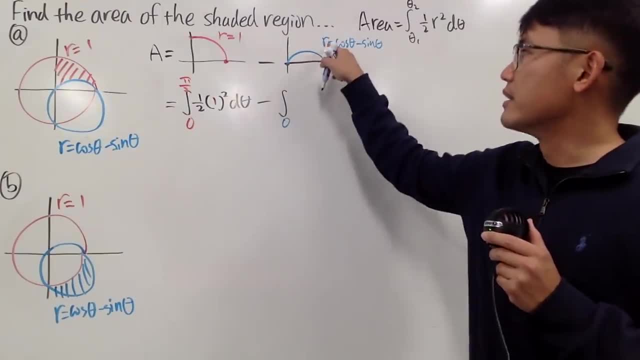 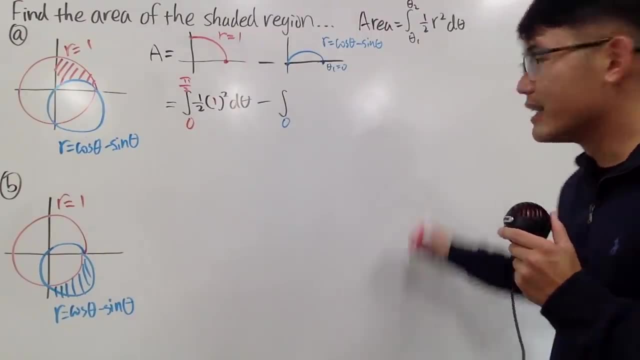 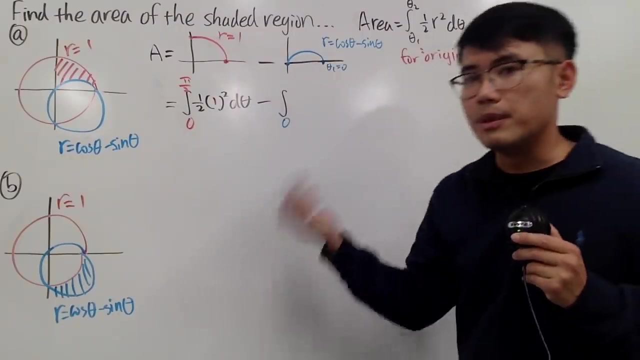 we are at the origin, we have to make the r equals zero. so we will just have to do that, and let me just put that down right here for you guys. so again for the origin, right? well, you can also call this to be the pole. that's why it's called the polar equations. 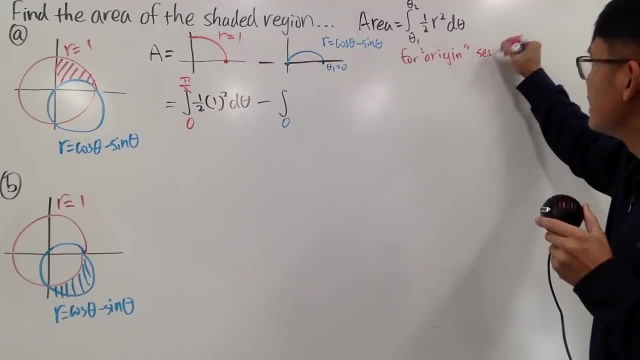 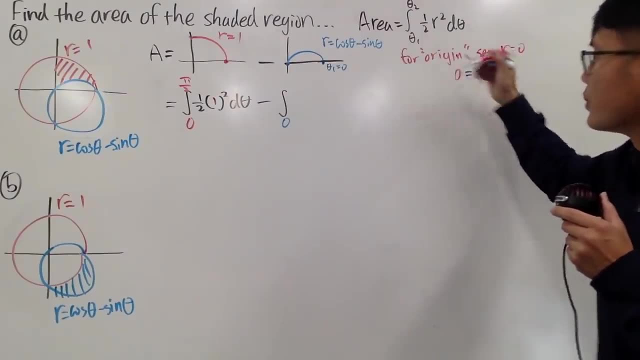 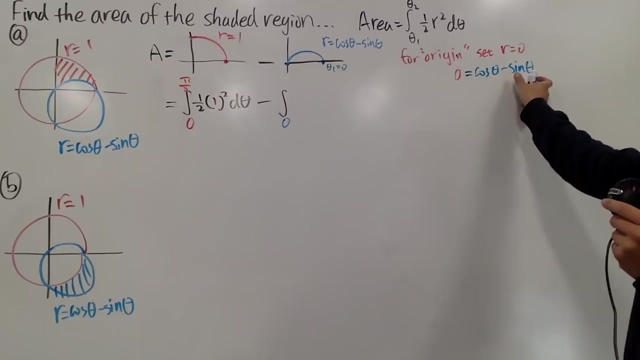 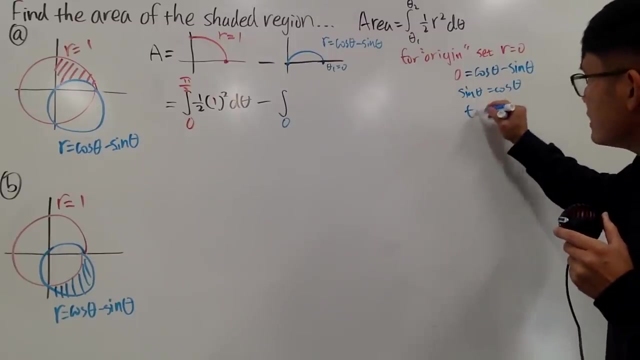 the polar functions. we have to set the r to be zero, so we get zero is equal to cosine theta minus sine theta. and of course we have to work this out real quick. bring the sine theta to the other side, so we have sine theta equals cosine theta. divide the cosine theta on both sides, we get tangent. 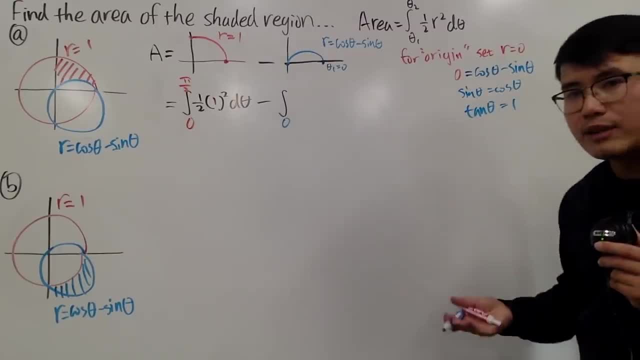 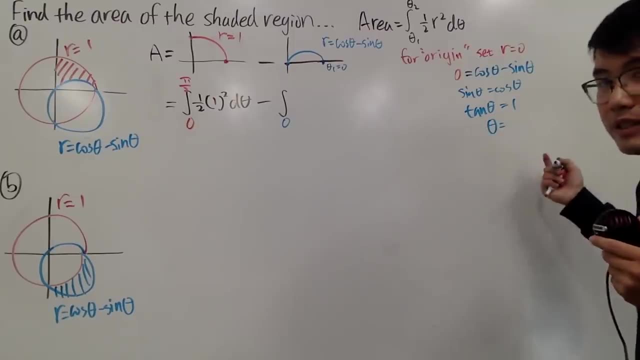 theta equals one, and now you just have to remember theta of theta of tangent of what angle will give us one? well, we have a lot of answers. the first answer is going to be pi over four, right, pi over four. and then the next answer is going to be phi, pi over four. 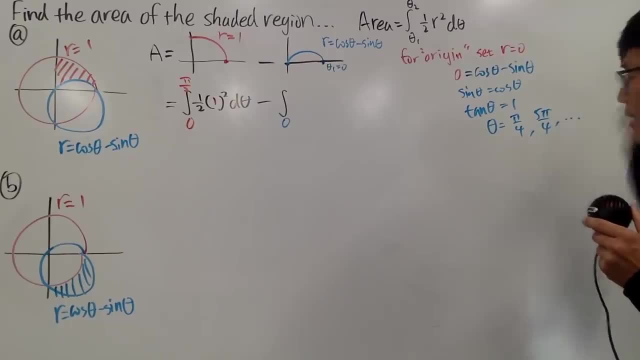 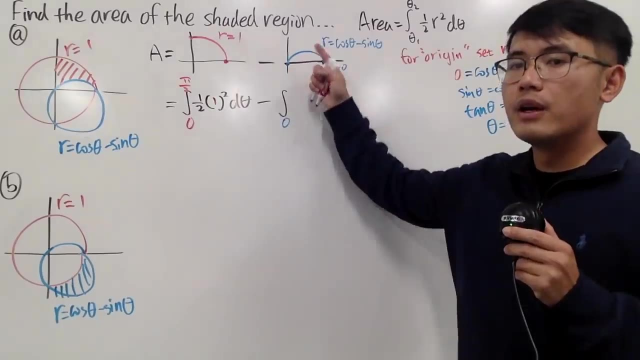 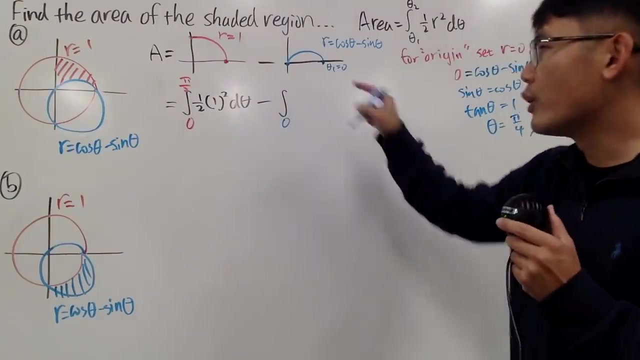 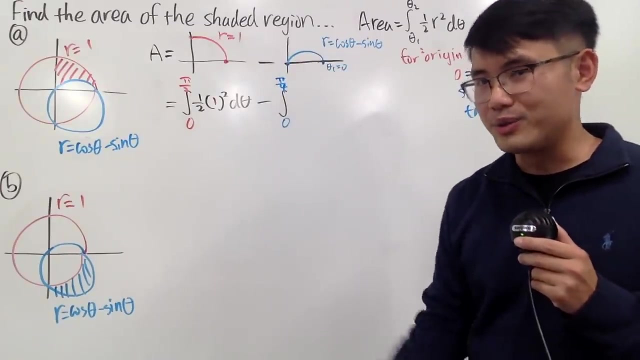 and of course a lot, a lot more. but you see that when theta is equal to pi over four, this is the first time that the curve hit the origin right, because when we have this angle, the r will be zero for the first time. so in fact it's actually at pi over four. if you plug in power four into thetas here, we will end up raised good zero. 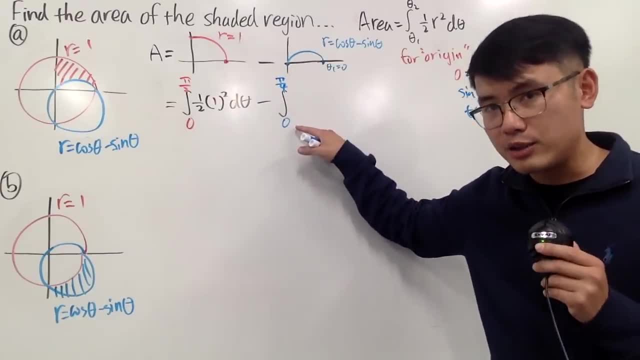 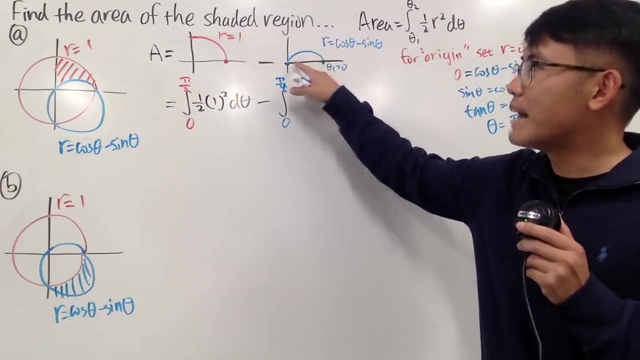 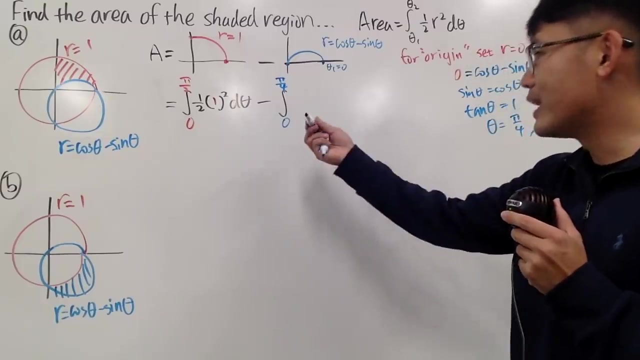 we will be right here. so you also have to pay attention to your starting and also your end, because our starting is, as you roll right here, we have to look for the first time that the r is zero. so this is a theta one, this is the theta two, and now we can just go ahead and put down the formula. 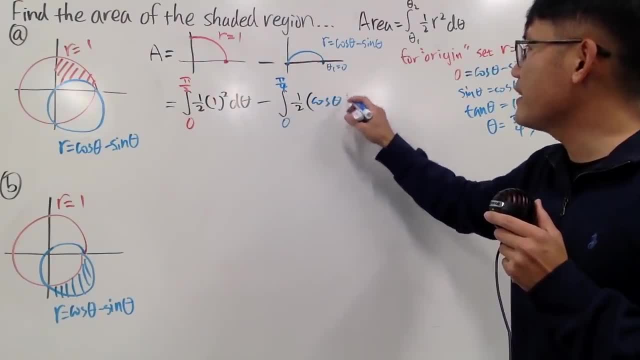 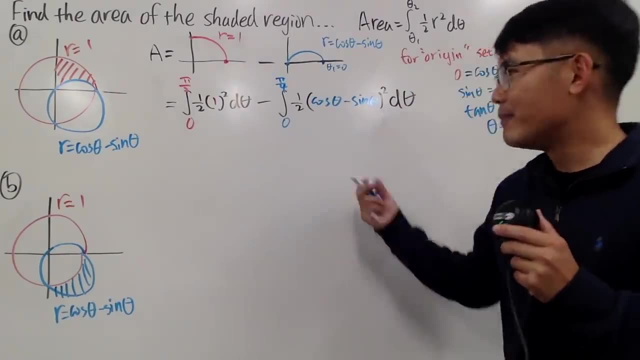 one half parentheses, with this being the r. then the cosine theta minus sine theta, don't forget. you square that and d theta. And guess what? I'm not going to work on integral. You guys will just do whatever you guys would like. 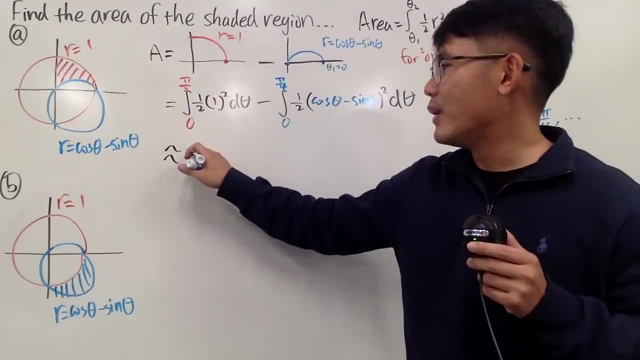 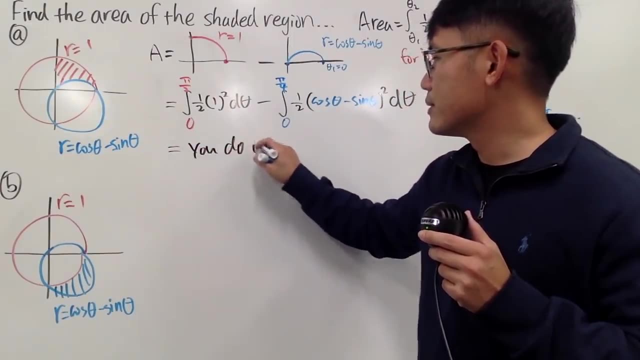 You can do this by hand, or you can use a calculator, and I will, you know, leave that to you. okay, It's just like you do it. okay, Don't write this down on the test. okay, If you write this down automatically, it's 0.. 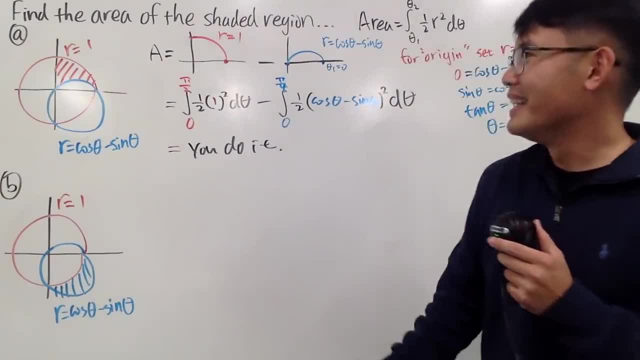 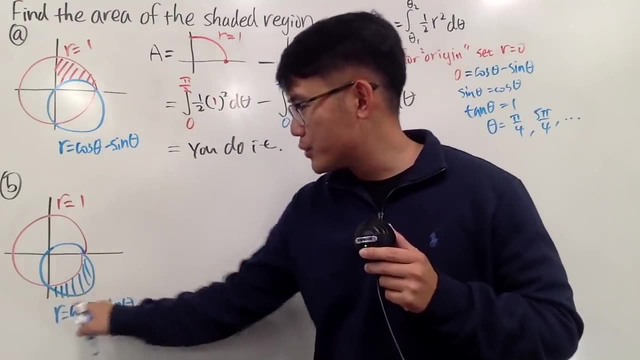 You have to actually do it and then put down the answer right here for me, okay. Anyway, let's look at the second one. Okay, for this one. hmm, it's different. huh, We have to go from here like that: the blue part and then minus the red part. 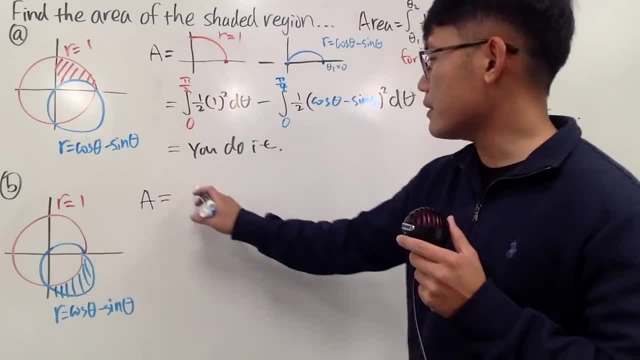 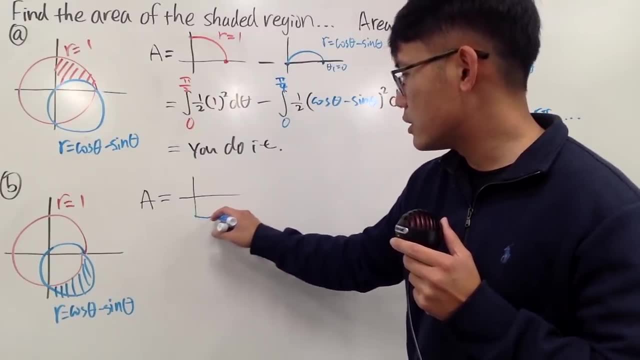 So I will just put this down right here for you guys: Area is equal to. we have to look at the blue part, which is like this: right? So this is not really like a quarter circle, right? This is the blue part, is not a quarter circle at all. okay. 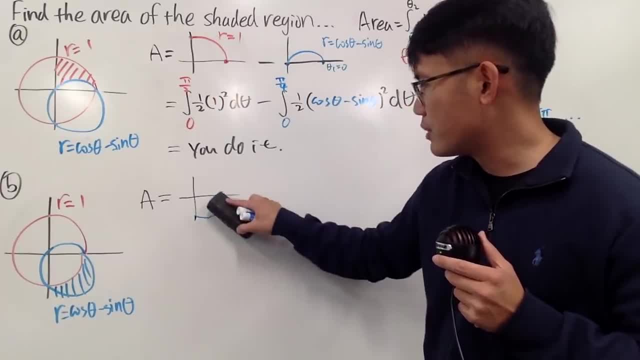 It's not a quarter circle. It's not a quarter circle at all, So just keep that in mind. My picture is not great, but you guys can see the better picture in the thumbnails. So this has nothing to do with quarter circle. 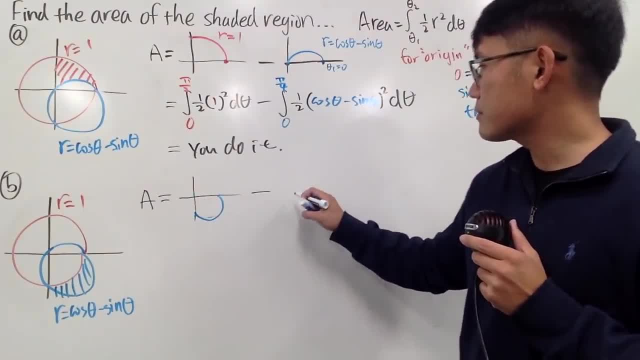 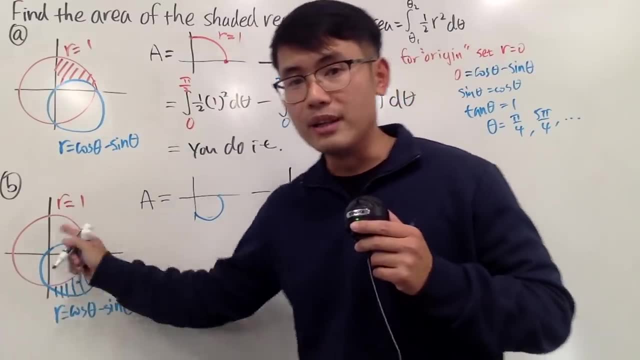 So we have to do this part and we have to minus the red part. The red part is a quarter circle, so that's very nice. Why? Because the origin is at 0, and the radius is 1.. So that's good. 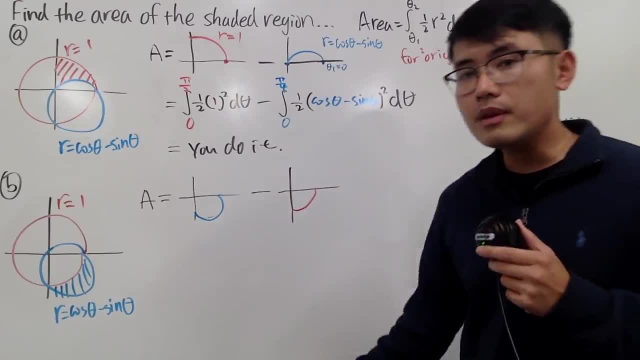 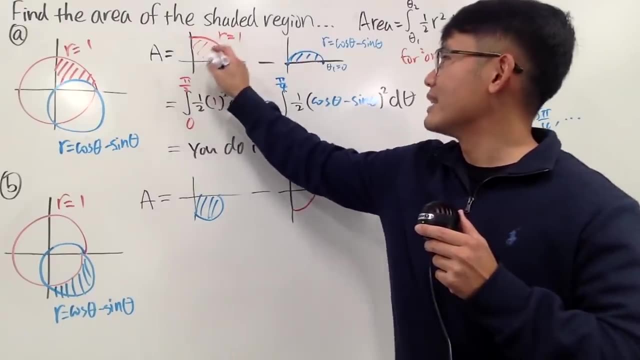 And now let's see, this is the quarter circle. I forgot to color the regions. Okay, So we have this and earlier we have all that. So just do some geometry and all that. Okay, here we go. If you would like, you can do the easy one first. 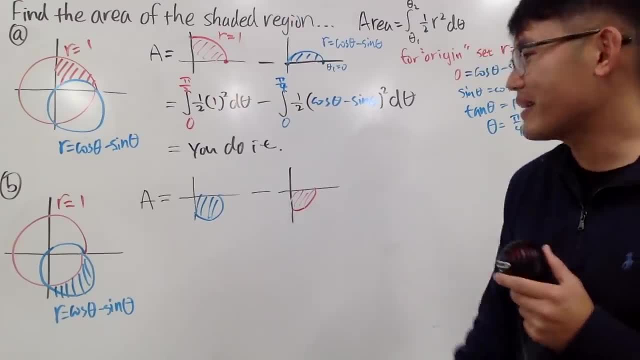 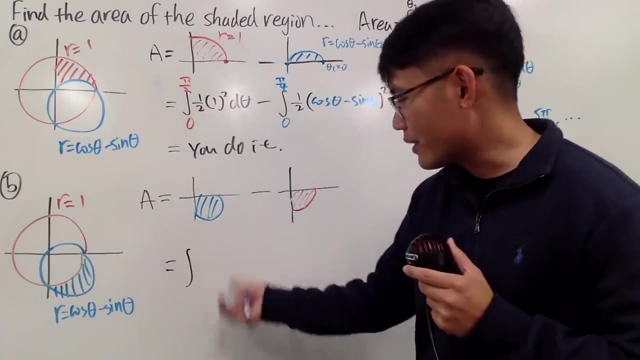 From 3 pi over 2 to 2 pi. done fine. okay For this one. let's face the reality. We have to do the hard part. If you would like, you can make some progress by putting down the 1 half and you square. 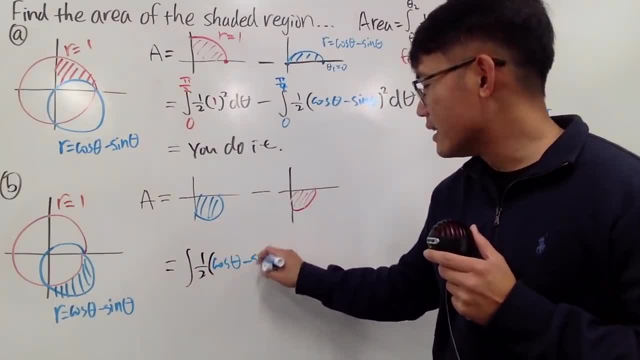 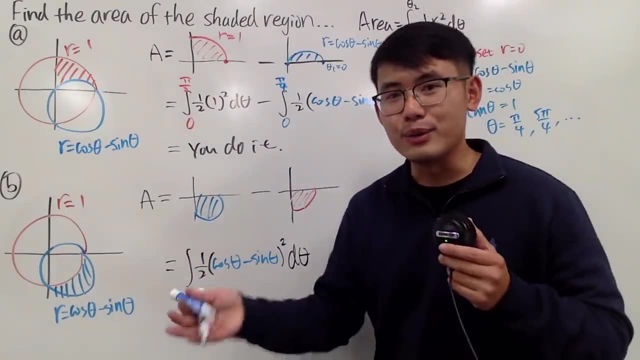 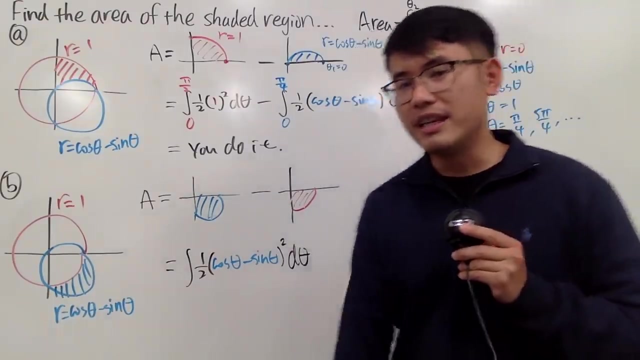 the r, which is that cosine theta minus sine theta, and you square that d theta. Okay Done, But without the limit of integration, I don't know. Okay, here is the deal. Perhaps one of the biggest common mistakes is the following: 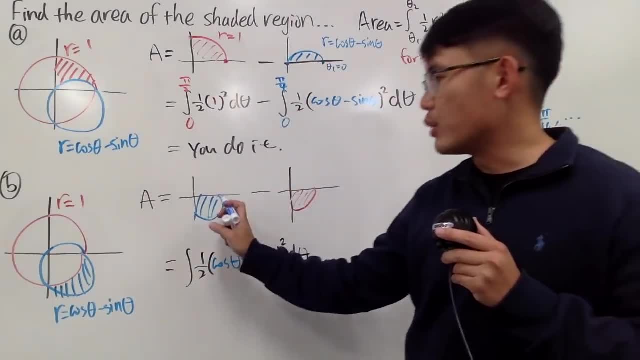 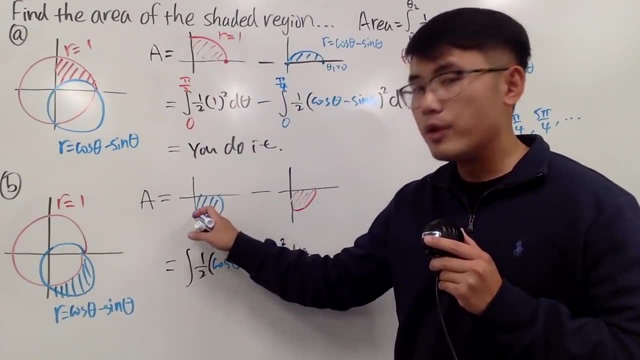 Of course you guys can see earlier we went from here to here, So you can see the orientation. it goes this way. So we have to start right here. We have to figure out for what angle will the curve hit this right here, right. 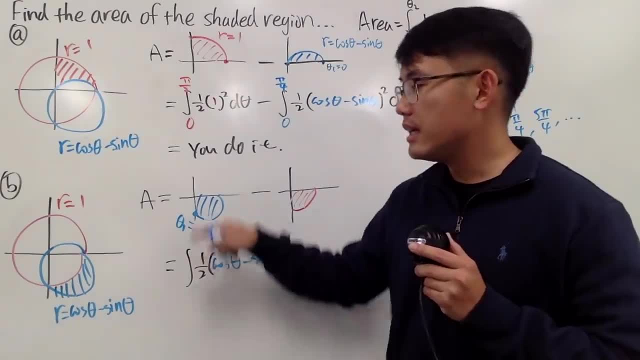 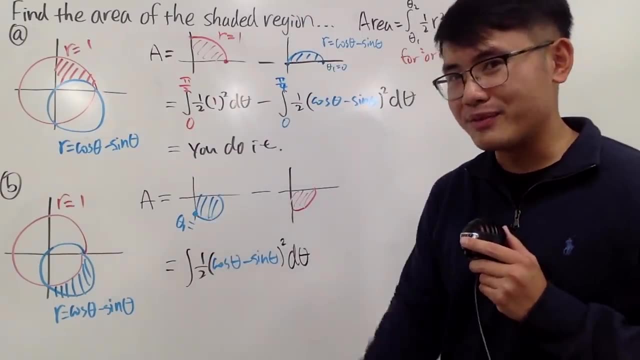 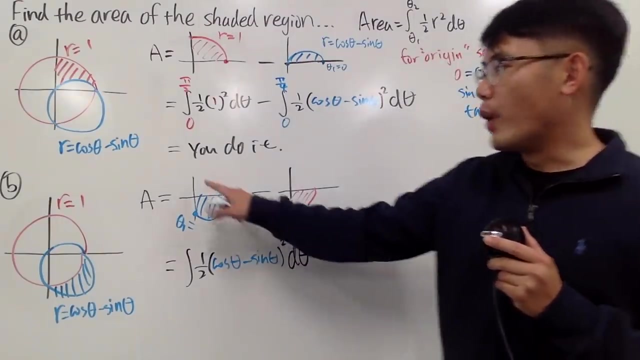 So that will be theta 1.. But This right here is actually not 3 pi over 2.. This right here is actually not 3 pi over 2.. Okay, this right here is a trouble zone When you are on the y-axis. let me tell you, whenever we have the point on the y-axis, 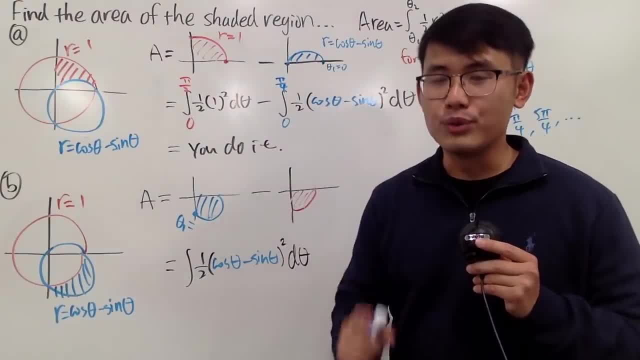 besides the origin, it's either you get pi over 2 or 3 pi over 2.. Keep that in mind. The best way is that just plug in to check right. So let me just do that for you guys real quick. 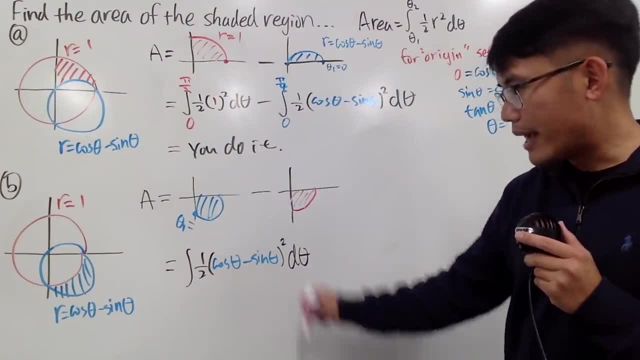 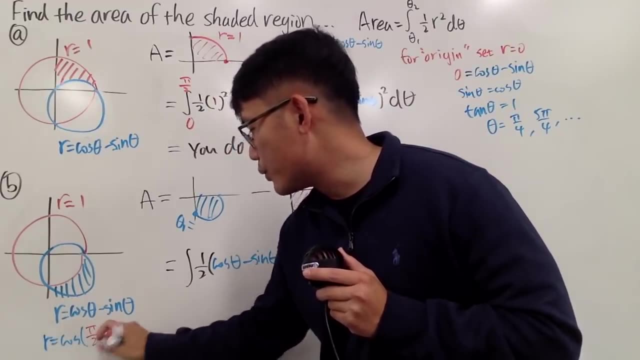 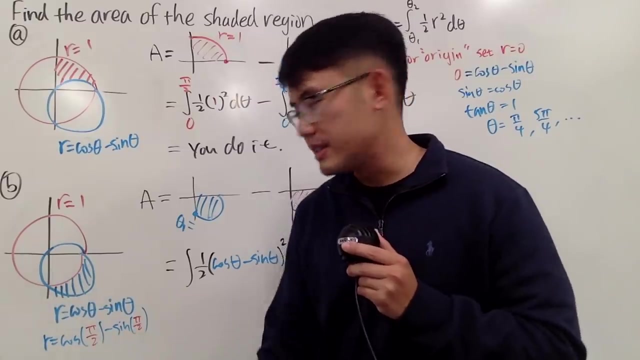 If our angle is at pi over 2, we will end up with: r equals cosine of pi over 2, minus sine of pi over 2.. Isn't it? And now check this out: Cosine of pi over 2 is 0, and we have: minus sine of pi over 2 is 1.. 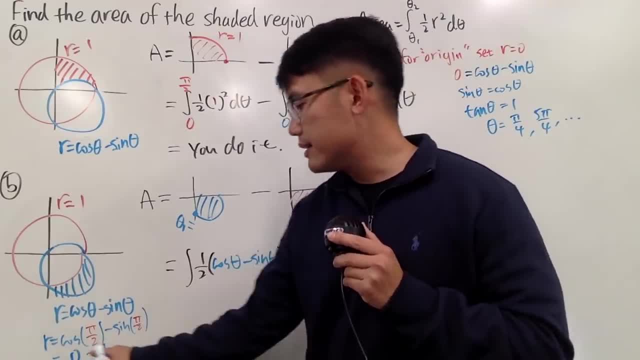 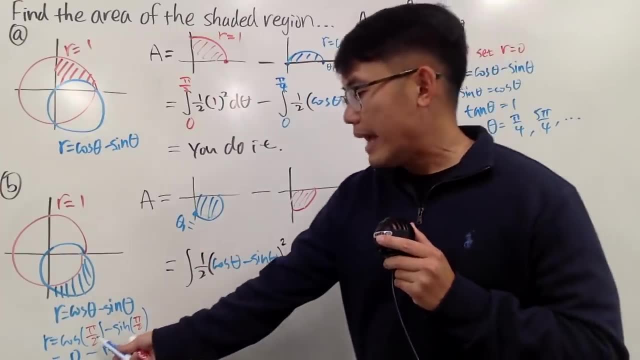 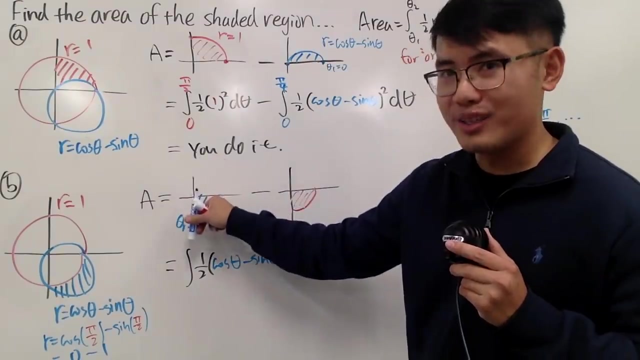 So in another word, r is equal to negative 1.. The two are equal Right Negative 1.. The truth is that for this point, well, angle is pi over 2, so we are looking up this way, But because r is negative 1, so we have to go down one unit. 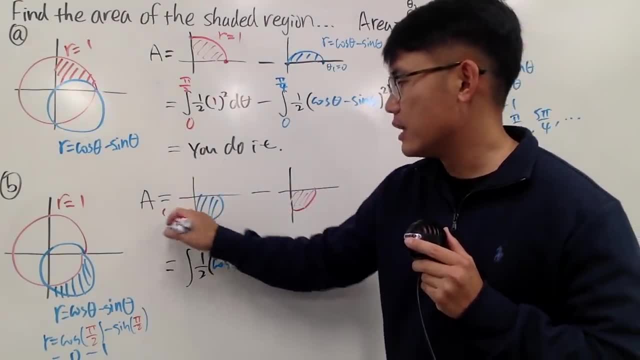 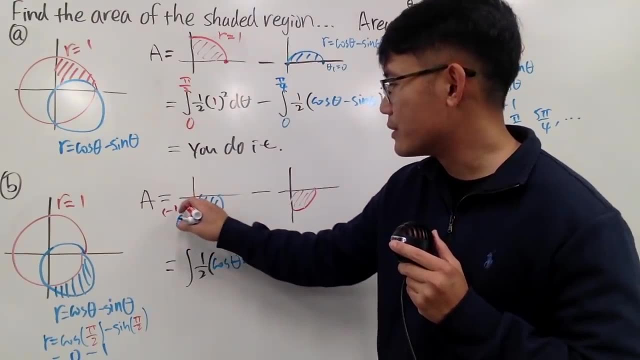 So the coordinate for this point is you write down the r first, which is negative 1, and you put down the theta, which is pi over 2.. And in fact this is the first angle that will give you this point on this curve. 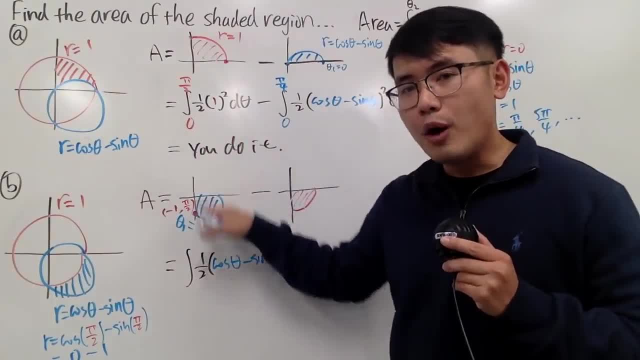 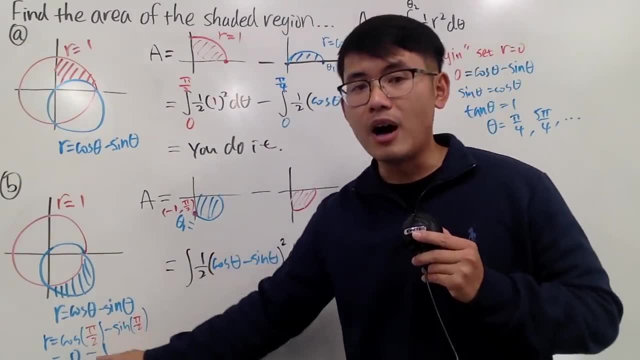 Pi over 2.. So keep in mind, whenever you are on the y-axis, the theta is either pi over 2 or 3 pi over 2, but you have to be careful. Sometimes the r might be negative. So even though you're looking down this way, huh. 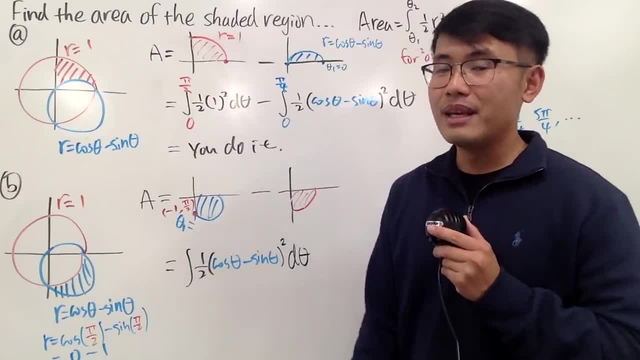 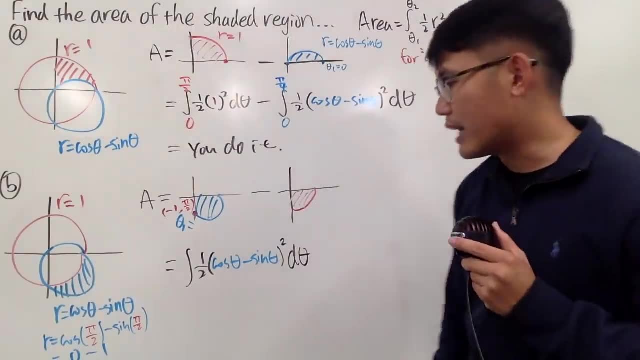 But it's actually pi over 2 because the r is negative 1.. Any point on the y-axis besides the origin, of course, Origin is always going to be when r is equal to 0, so you have to do that. 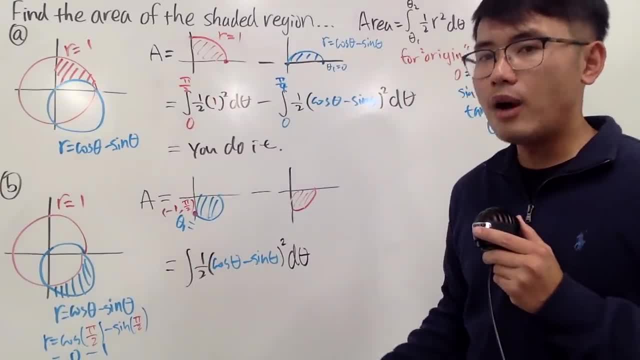 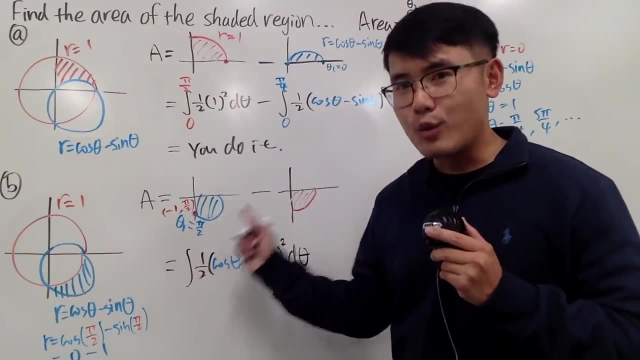 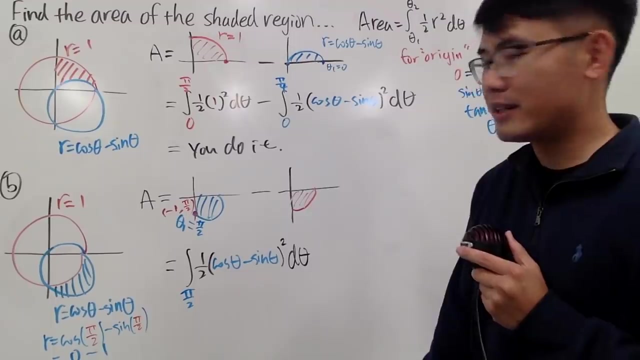 So theta 1 is pi over 2.. So let me just put this down right here for you guys. This is why I did the graph by hand with my students in class, right? That's why you can feel about how to graph all these things much better. 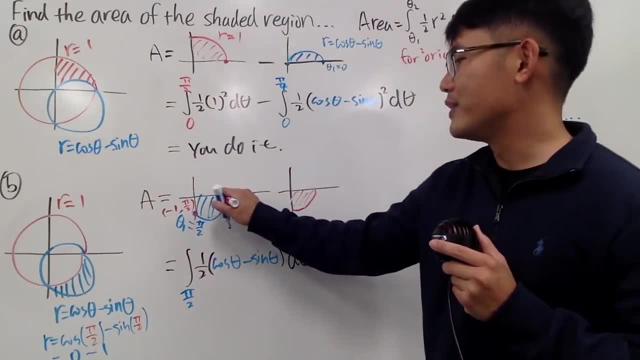 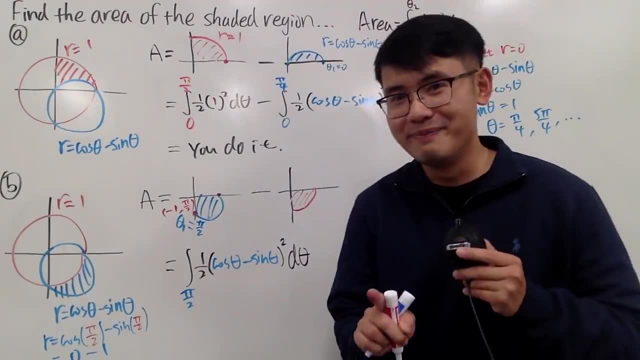 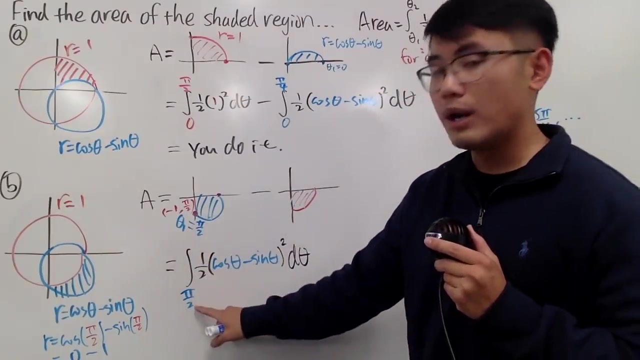 And now, similarly, we have to figure out for what angle will give us this point, Even though we're looking at this direction. but it's not 0. This, right here, the theta is not 0. Because we started at pi over 2 as our theta 1.. 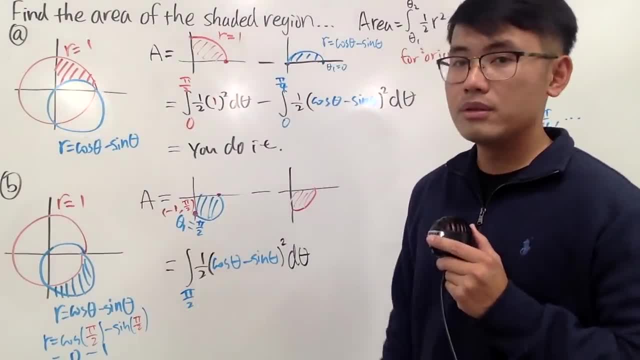 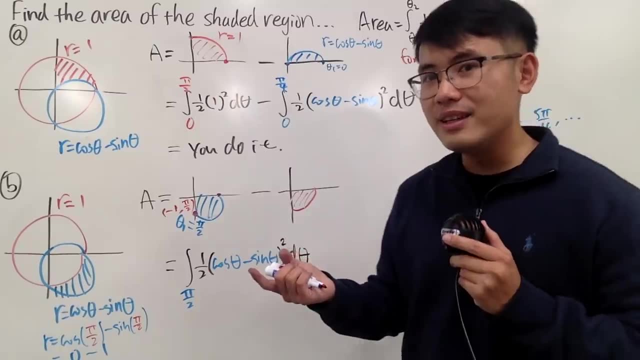 This point. this number here has to be bigger than pi over 2.. Okay, keep that in mind. Well, similarly, this point is on the x-axis, So theta is either going to be 0 or pi. Of course, you have a lot more like 3 pi, 4 pi and so on. 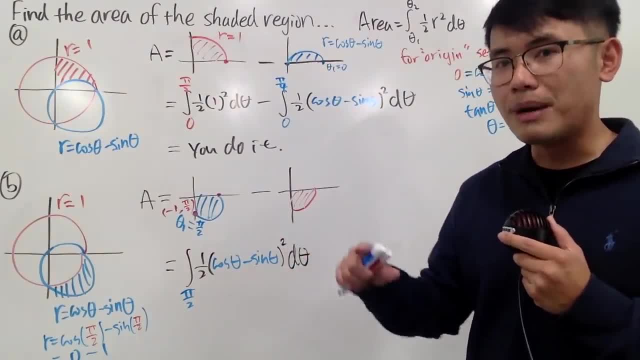 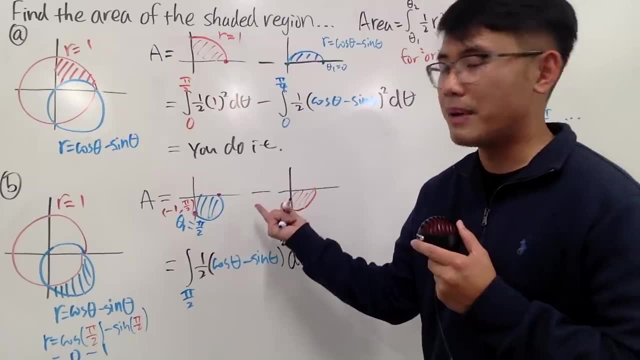 2, pi, all that, Don't worry, either 0 or pi, That will be the things you should use first. And because we have pi over 2 already, you can kind of guess that this is actually pi, Because this number for the theta has to be bigger than pi over 2.. 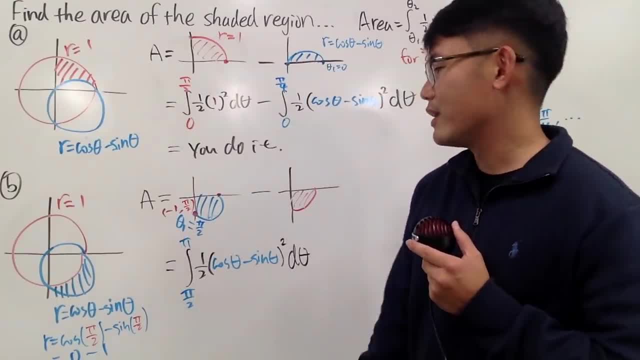 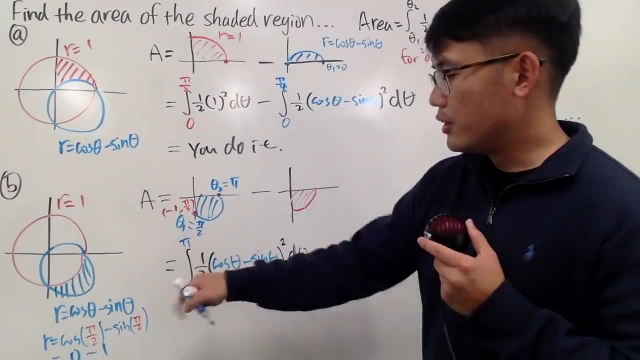 I'll put on pi right here for you guys. first. It's actually the answer. It's pi Why? Because let me tell you, if you put in theta 2 to be pi, if you put on pi over 2, I mean pi right here. 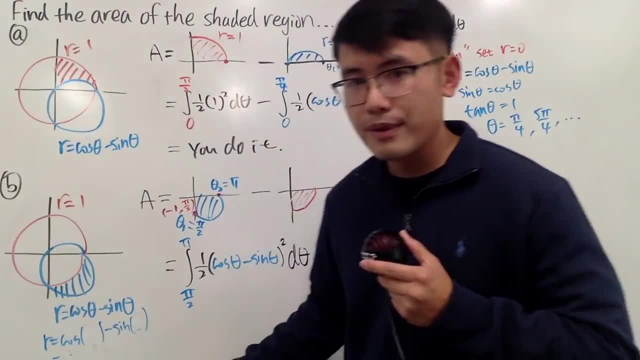 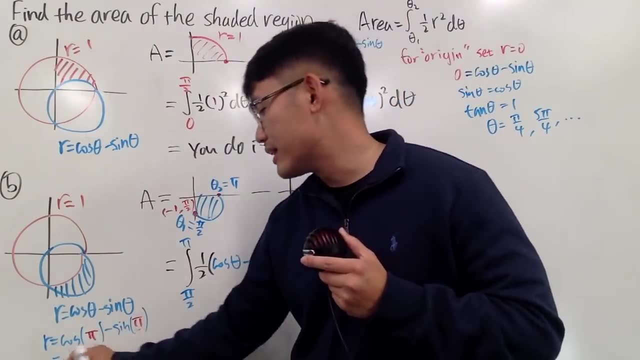 Let me just erase this real quick. When theta is pi, you put on pi here and pi here, Cosine of pi is negative 1. And then sine of pi is 0. So, yes, again we end up with r equals negative 1.. 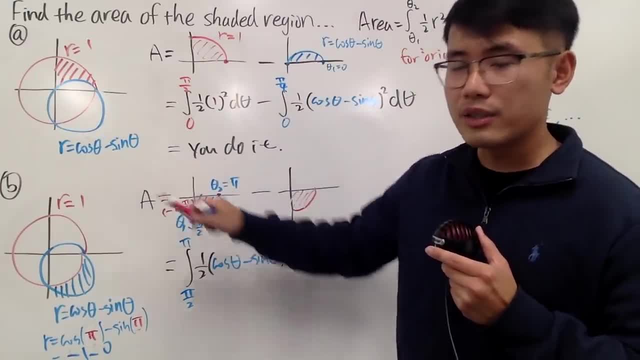 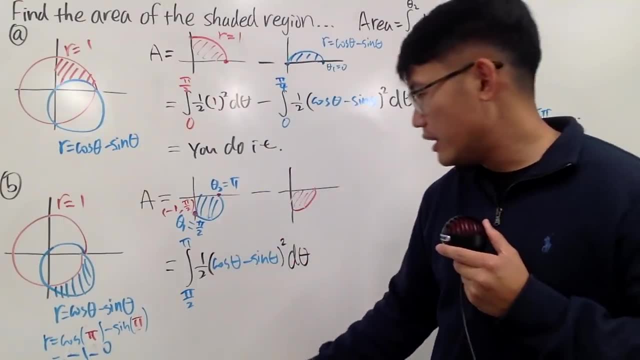 So the angle is pi, which we are looking at that direction, We're looking at this direction, But r is negative 1, so you go back one unit, So hit this In another word: this coordinate is negative 1, pi. 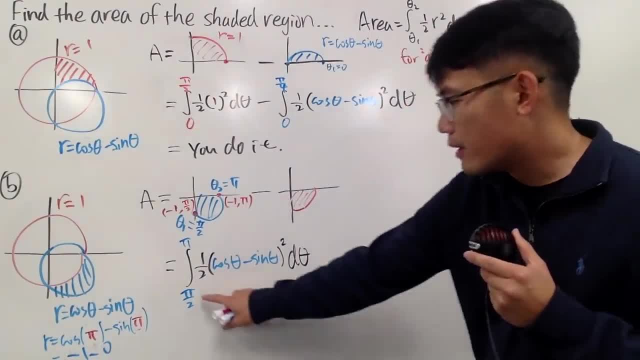 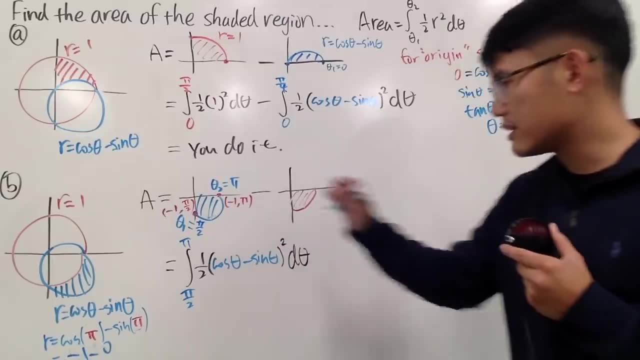 It's on the x-axis. Okay, So from pi over 2, the next theta for you, which is going to be pi, You don't do 2 pi. You don't do pi whatever. That's the idea. 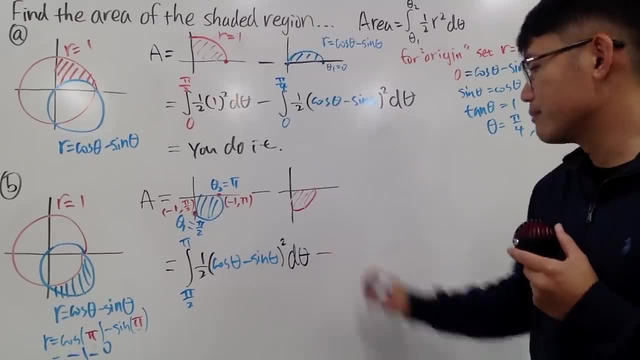 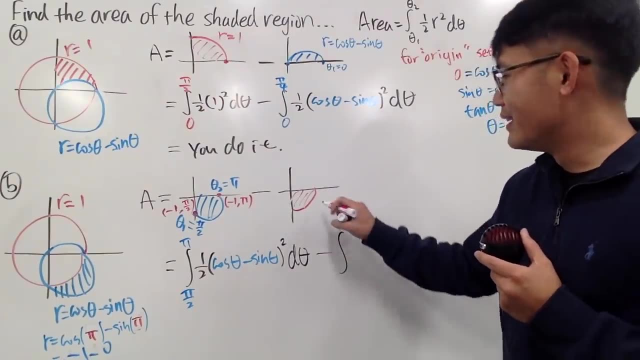 So that's it, And then you pretty much do this Minus integral For this right here. it's not that bad at all, because r is always 1.. Right, This right here, r is always 1. So it's nothing tricky at all. 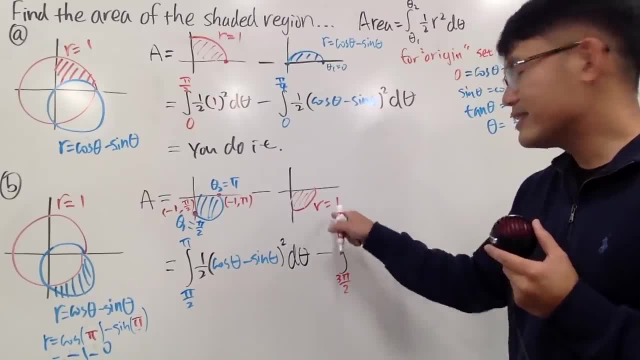 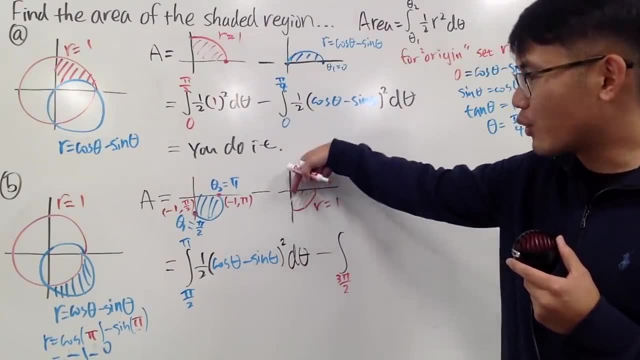 If you look down, this is just 3 pi over 2.. Because there's no way for r to be negative. r is positive 1 already. So you have to look down pi over 2 direction and then go forward one unit to reach this point. 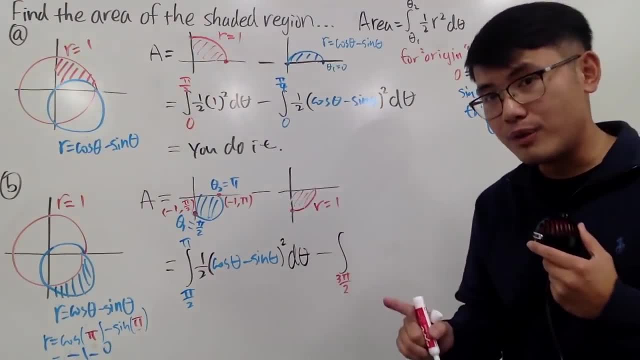 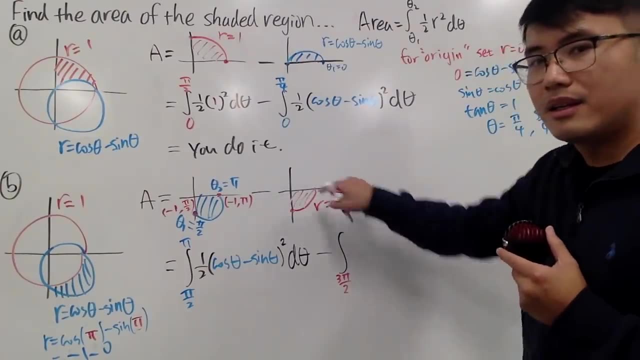 And then when you have this, you don't put down 0 because you have 3 pi over 2 already- You have to put down 2 pi. This is 0.. This is also 2 pi, This is also 4 pi, and so on. 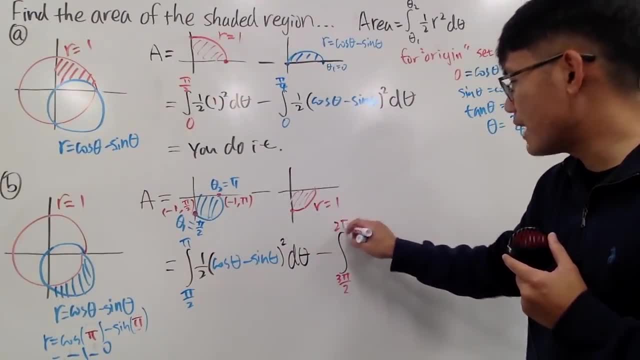 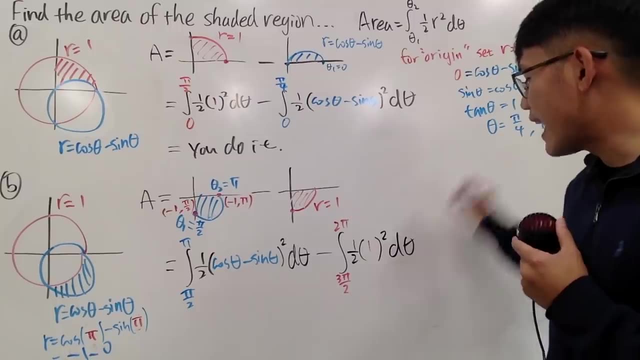 Right And you are going forward. So you have to put down 2 pi for this And of course, you put down 1, half r is 1, and you square that d theta. And again the answer to this right here is: you do it. 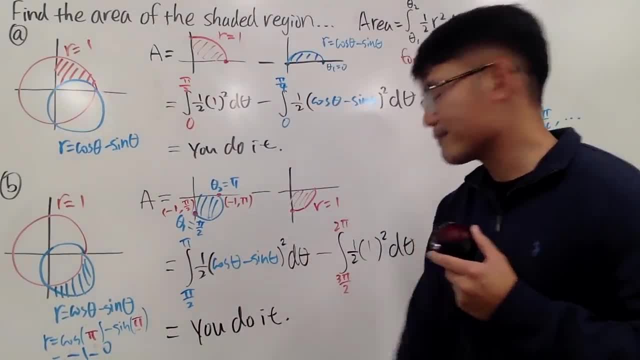 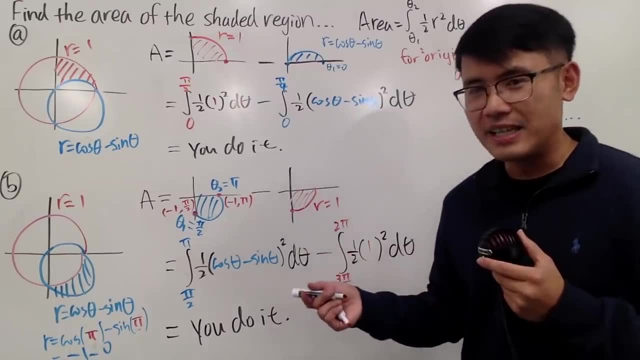 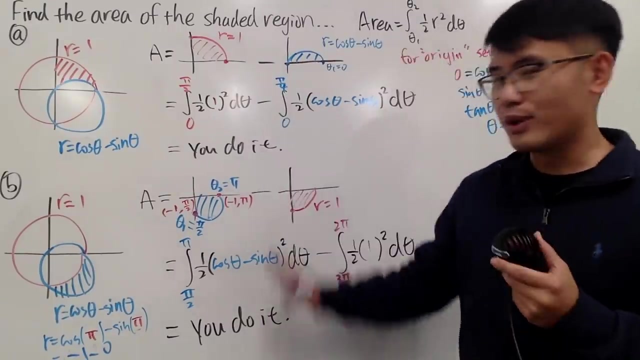 You do it. Yeah, I will be surprised if my students really write down you do it on the test. I will take a picture of that student's test and I will share with my subscribers. So if you are my students, seriously just don't do that. 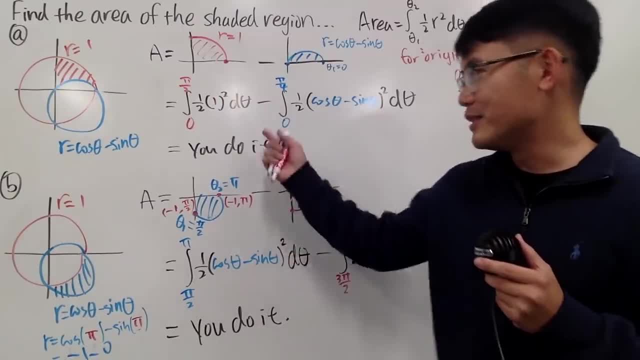 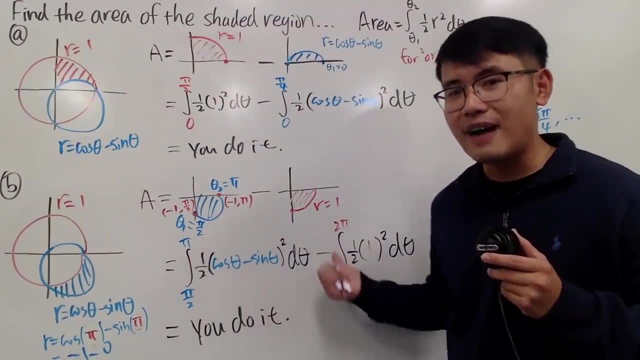 And if you are taking Cal 2 with other professors, seriously, don't do this to your professors. Seriously, just work this out on your own. My goal was to show you guys how to find the theta values, to find the areas for the polar curves. 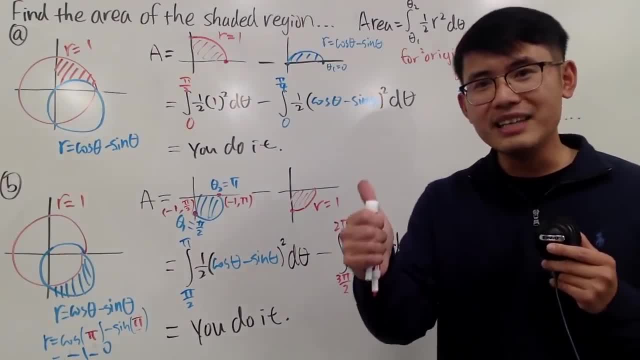 Right, Hopefully you guys all find this video to be helpful. Give me a like if you think so. Thank you guys so much. Welcome to the Property Management Basics session of the Property Management course. In this session, we will discuss what property management is and the various responsibilities that fall under property management. We will then identify why property management is important to investors, focusing on properties specifically buy and hold or lease to own. Finally, we'll